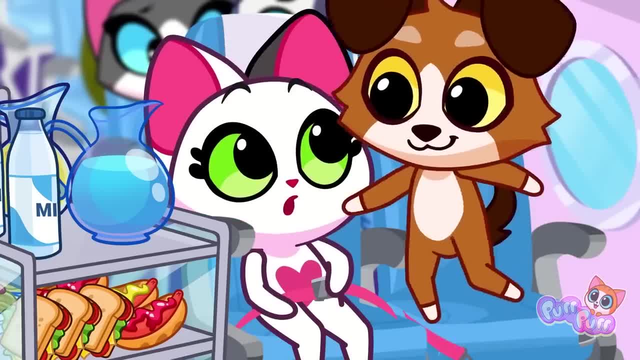 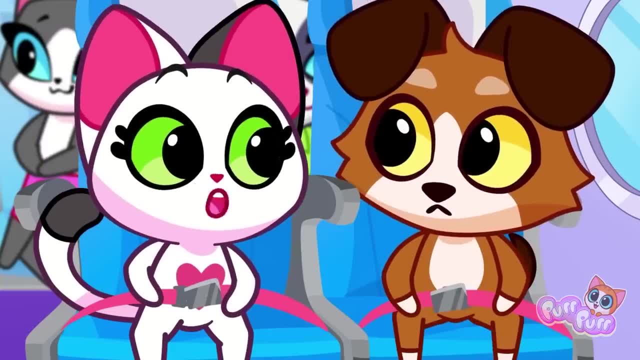 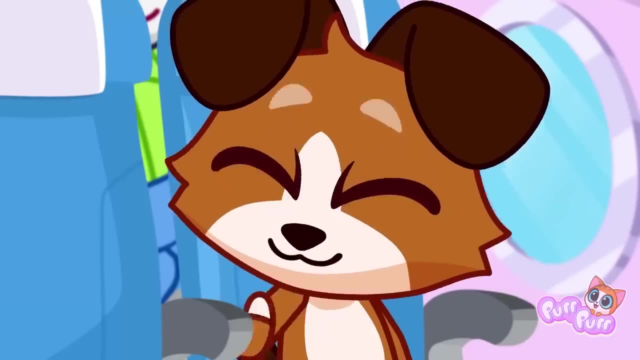 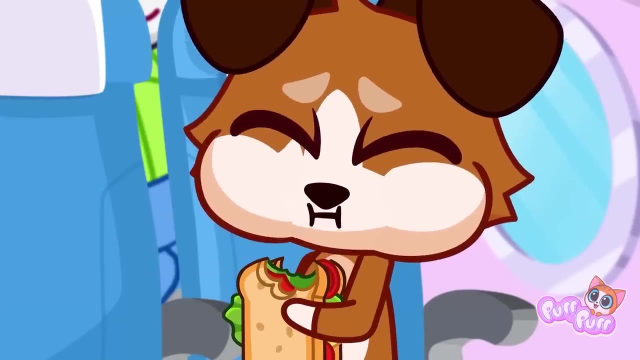 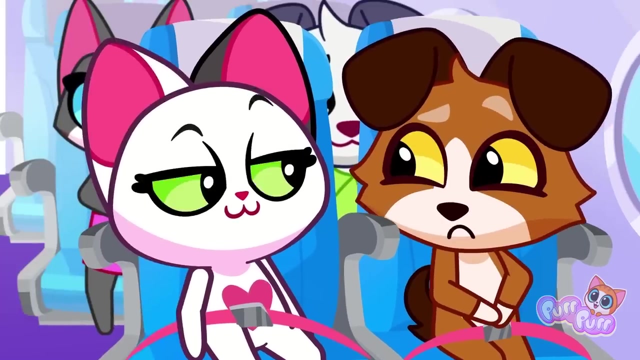 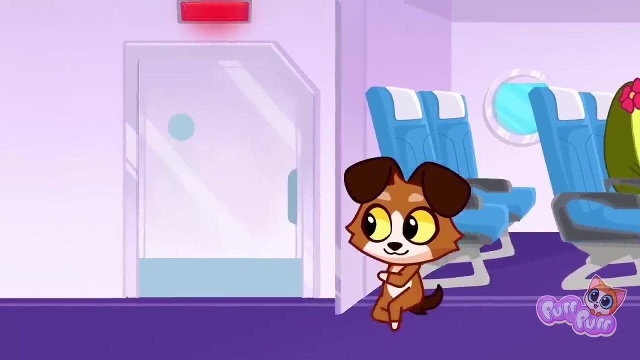 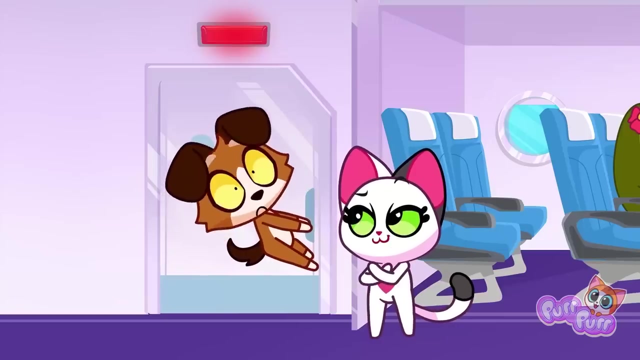 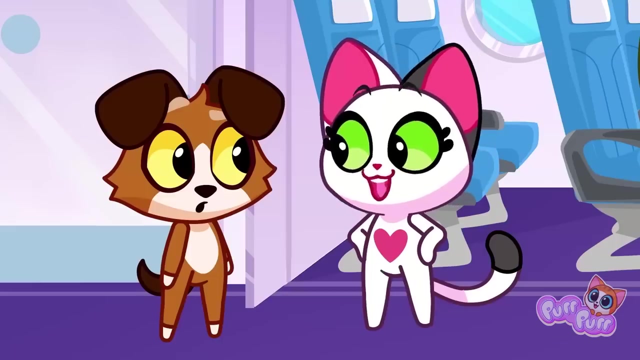 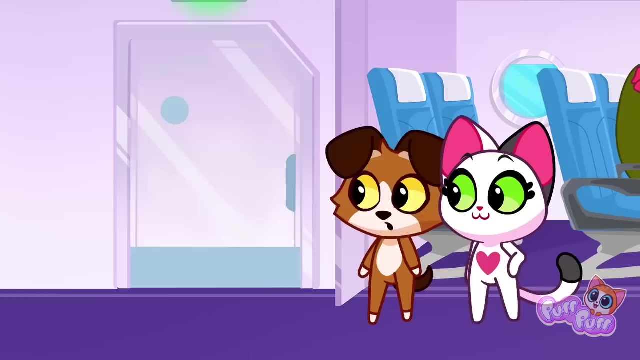 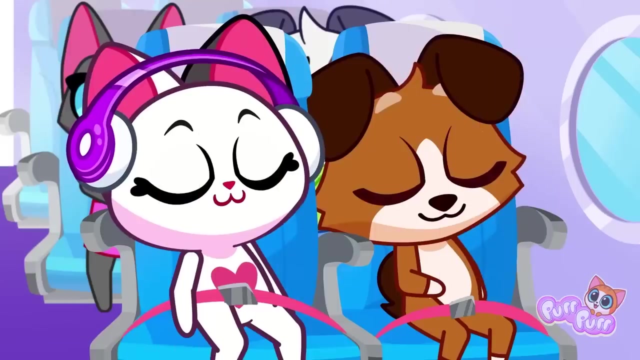 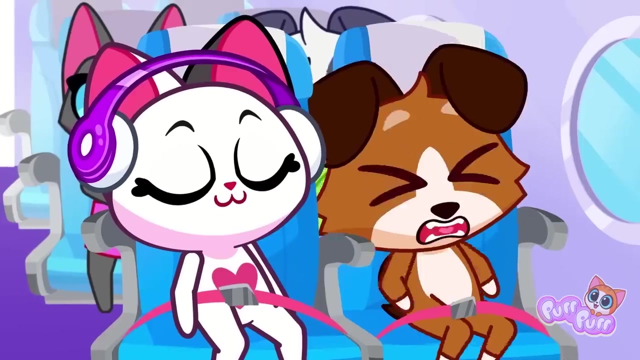 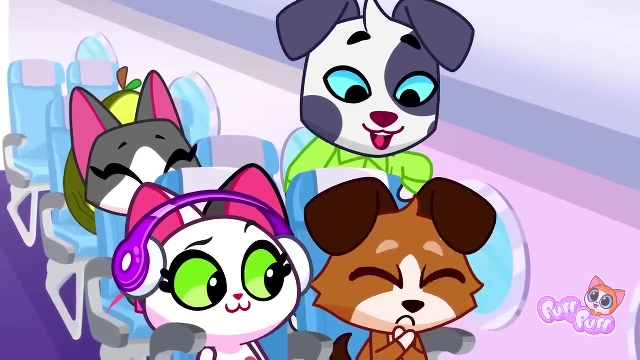 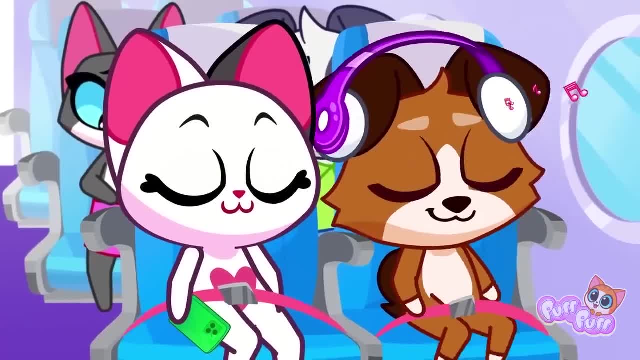 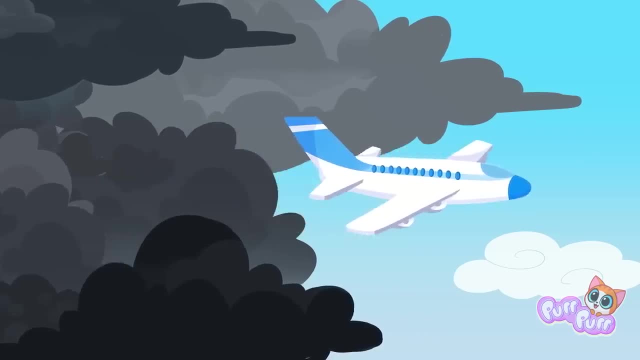 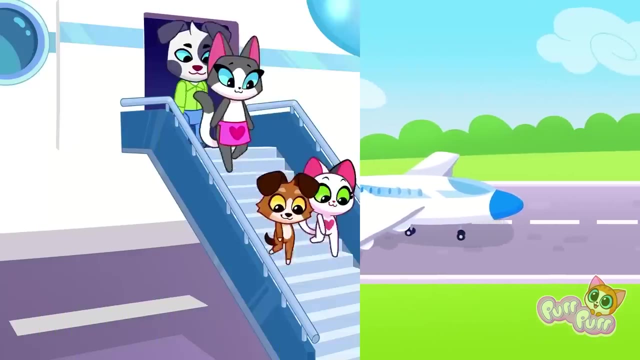 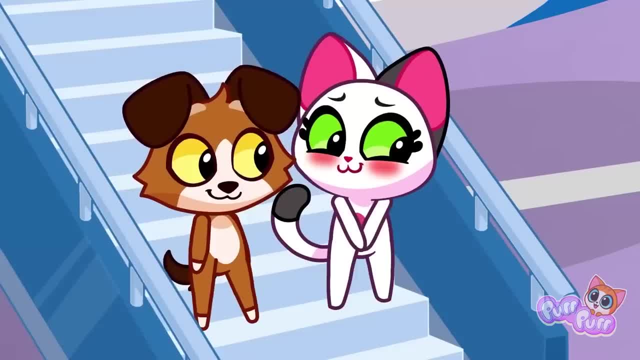 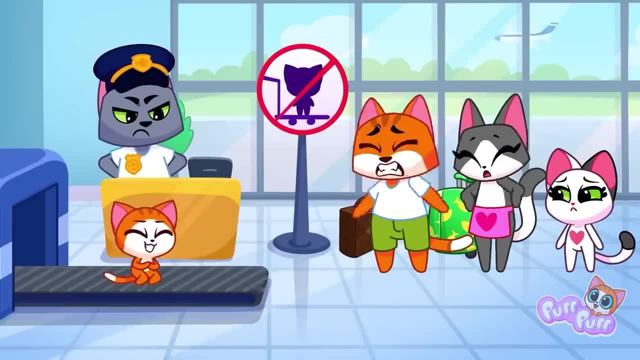 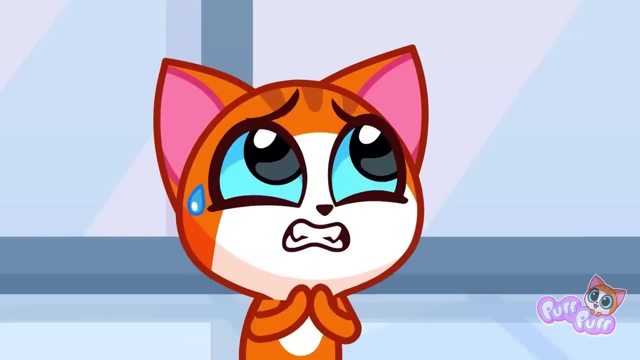 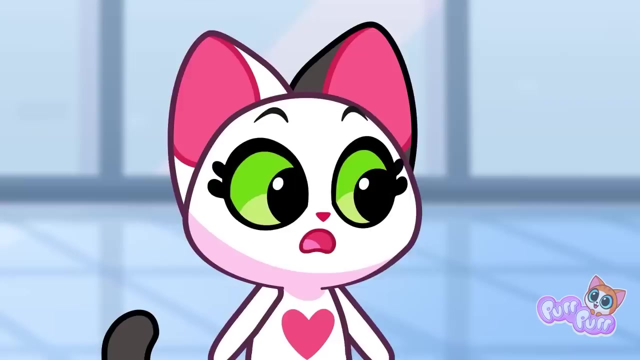 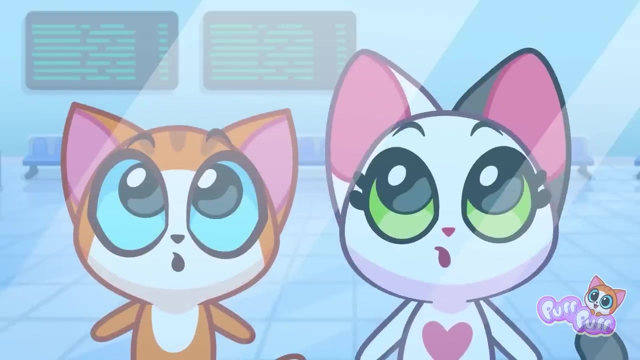 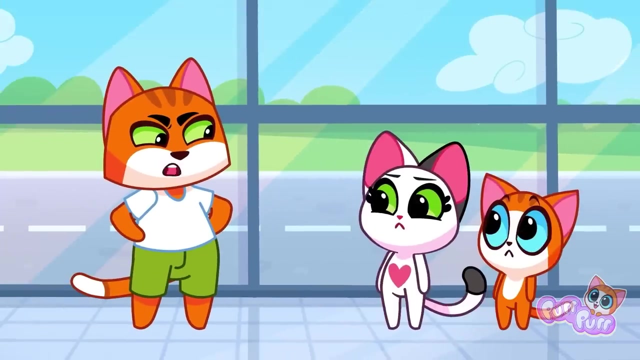 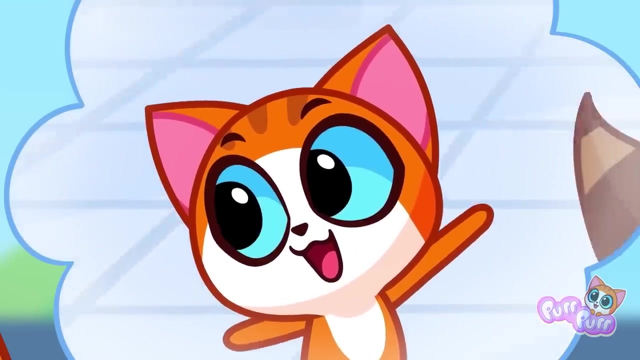 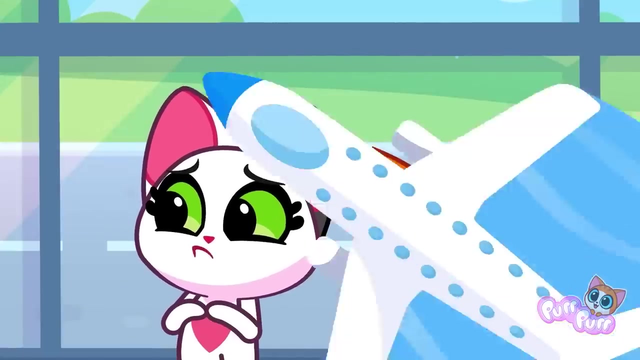 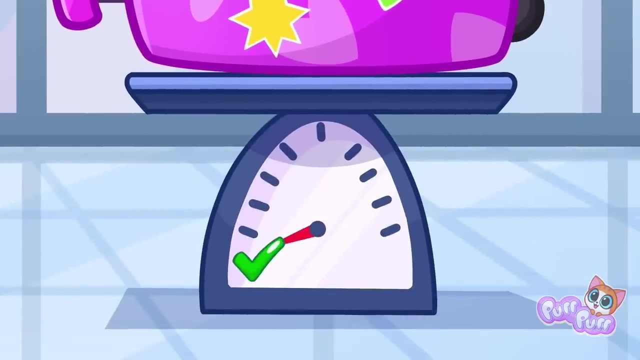 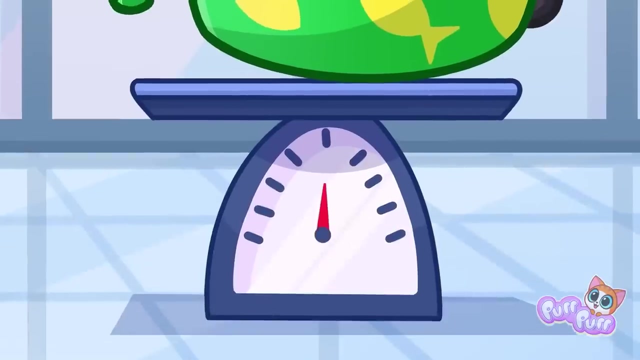 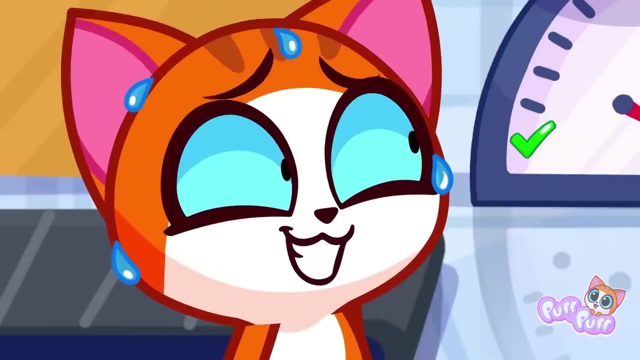 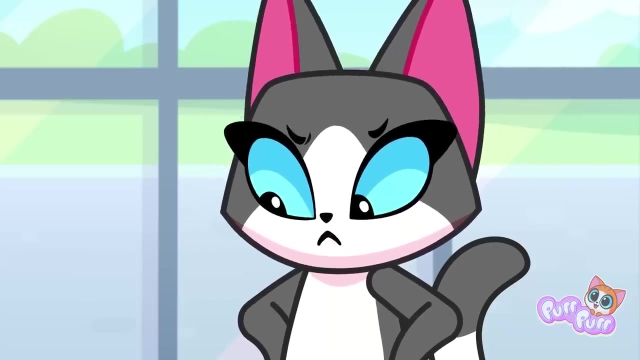 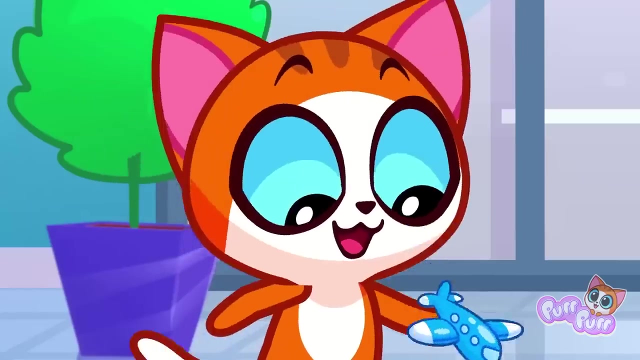 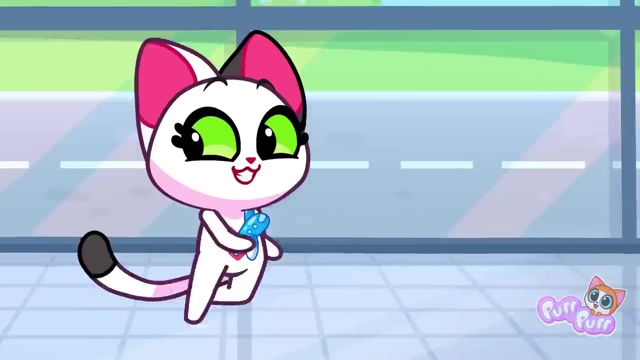 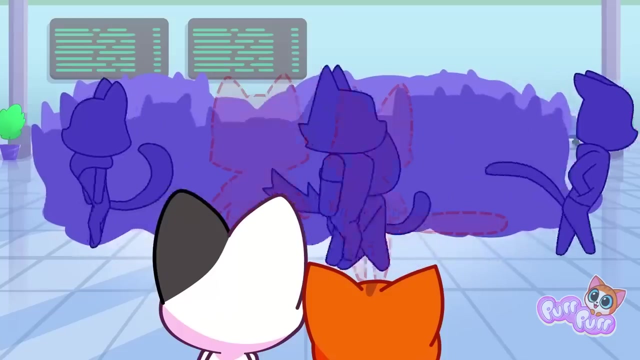 Thank you, Rock. Leo, you can't get on luggage tape. I'm sorry, Don't run away from us. It's easy to get lost here. It's easy to get lost here. It's easy to get lost here, Leo, you took too much stuff. Oh no, they left without us. 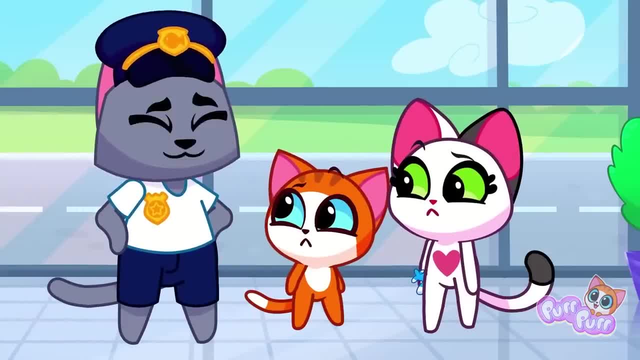 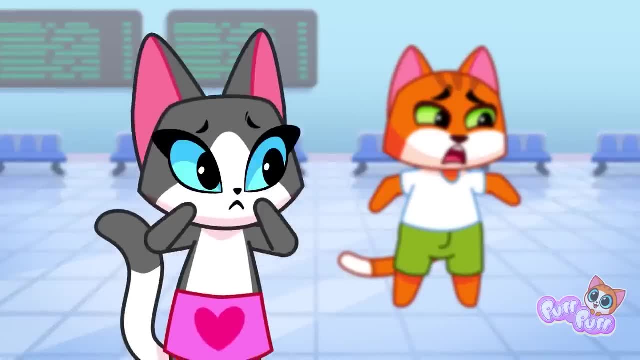 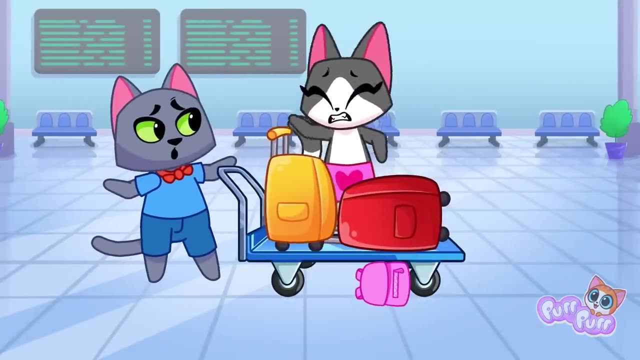 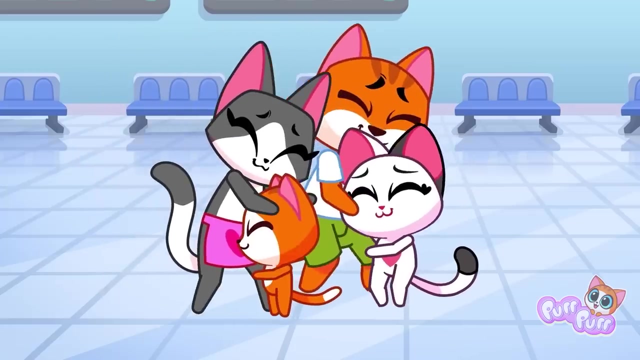 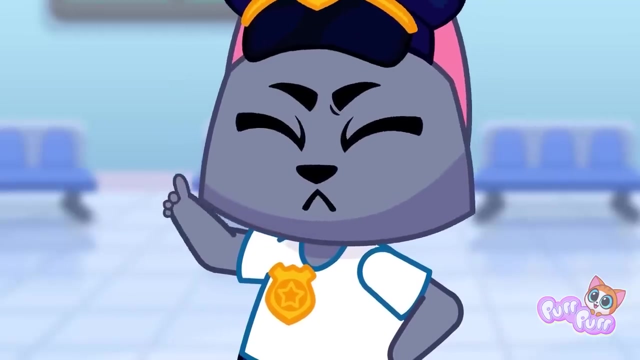 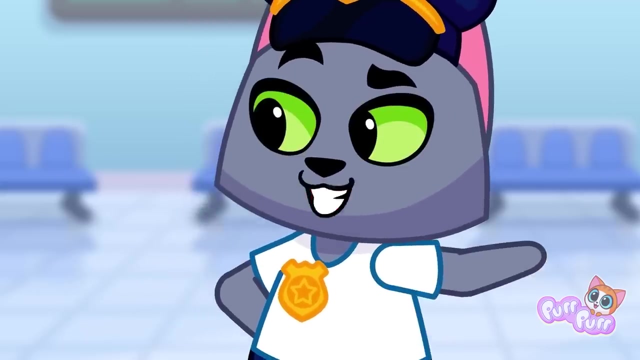 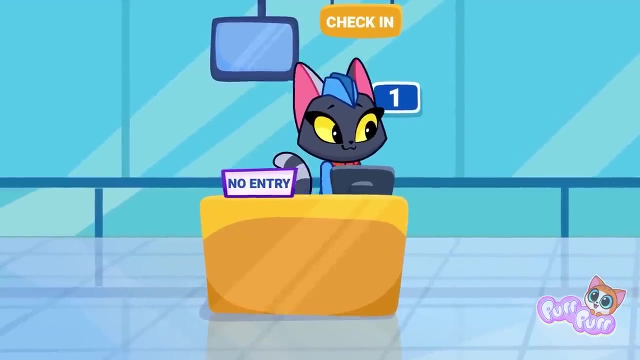 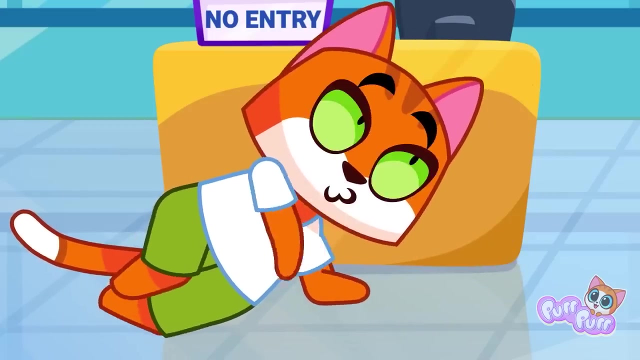 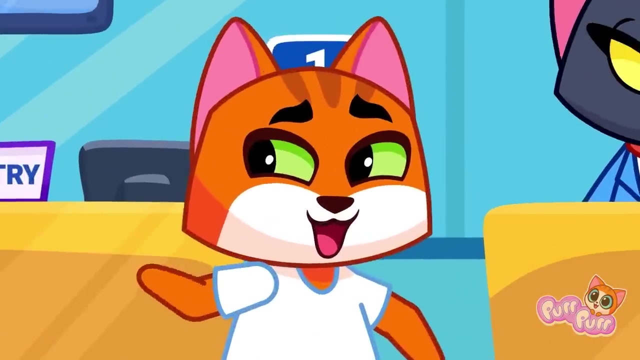 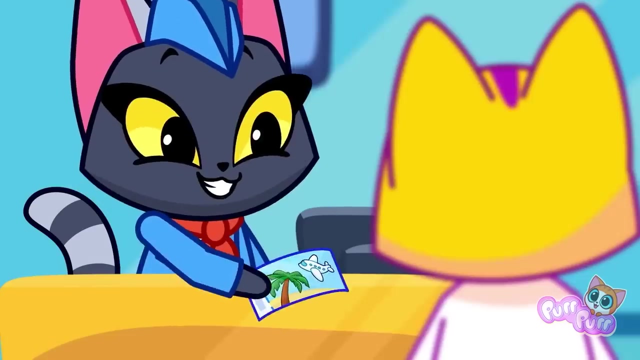 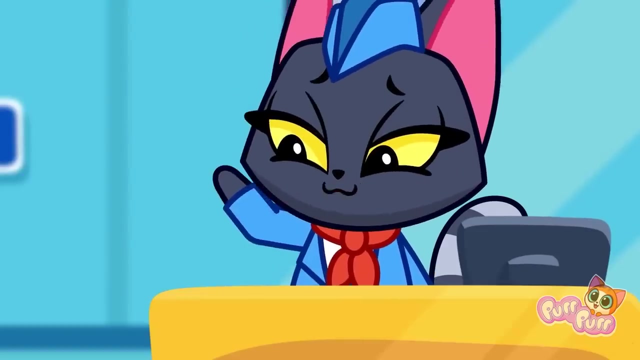 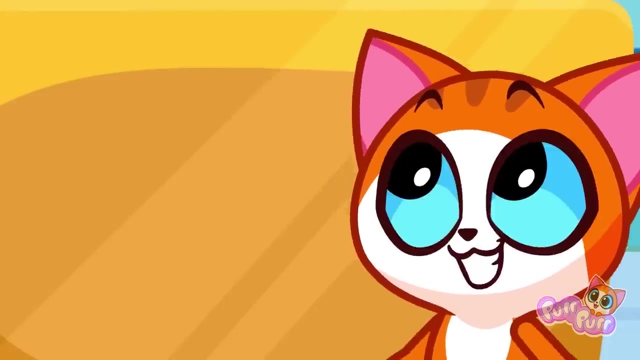 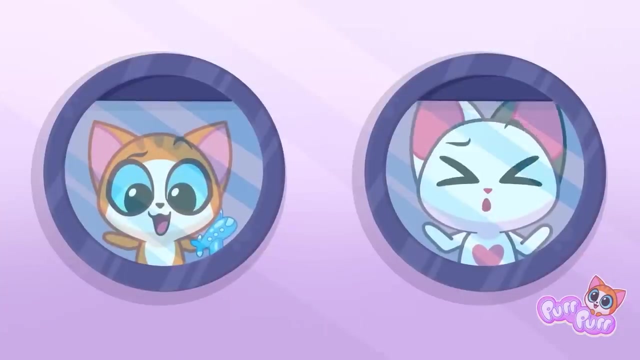 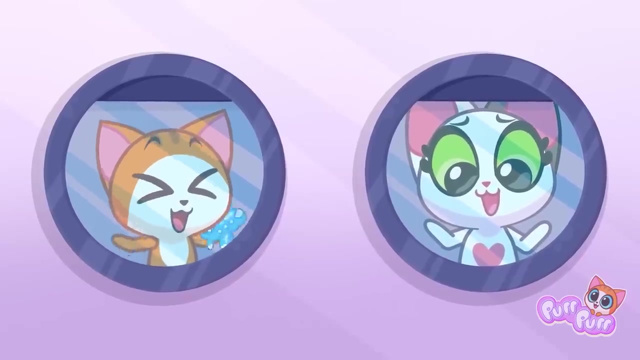 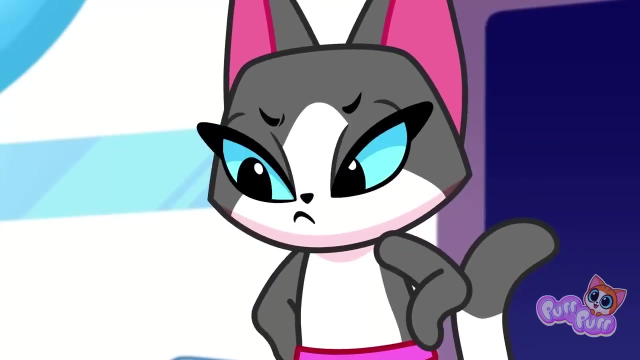 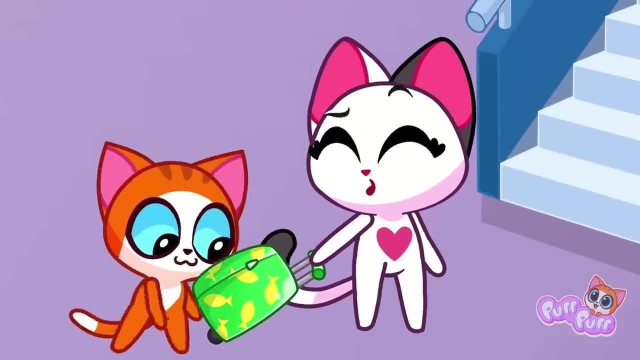 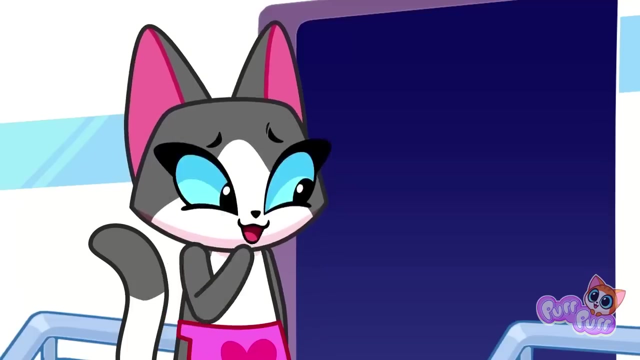 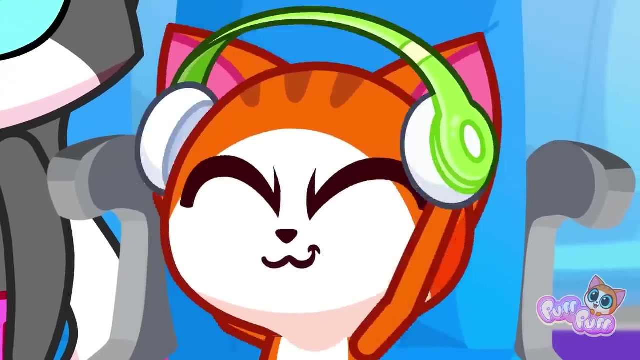 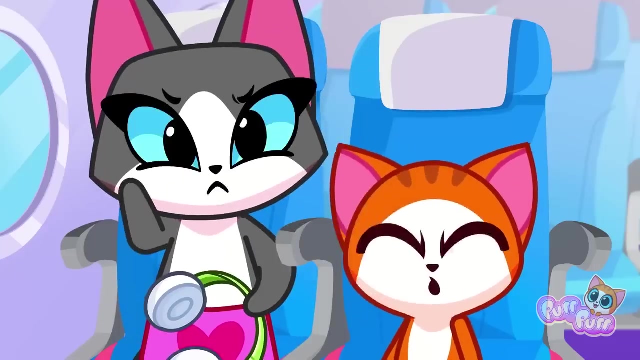 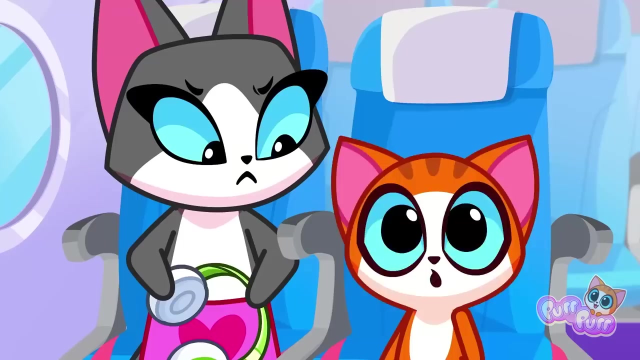 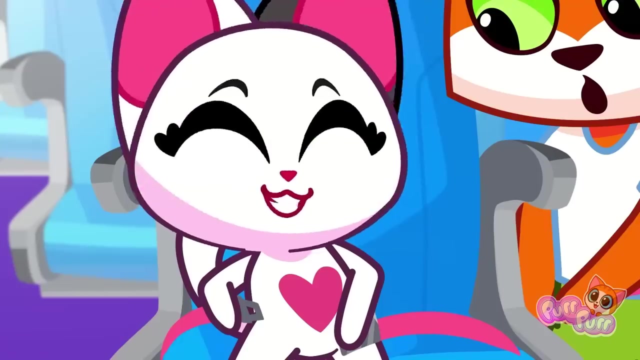 Kids, don't cry. I'll take you to your parents, Leo, Lucy, If lost, ask for help from a policeman or a stewardess. No way, No way, No way. It's important to keep the line. It's important to keep the line. It's important to keep the line. 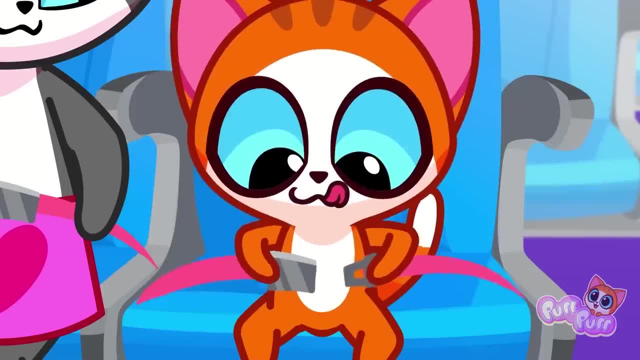 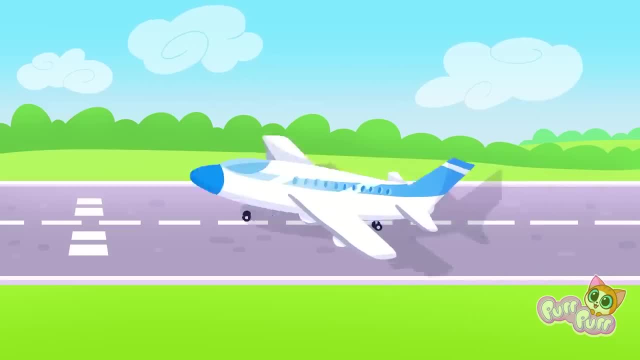 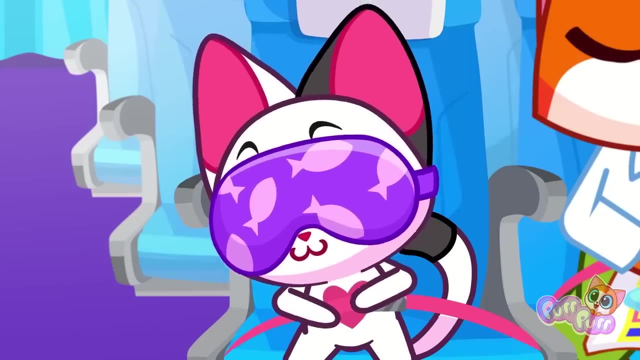 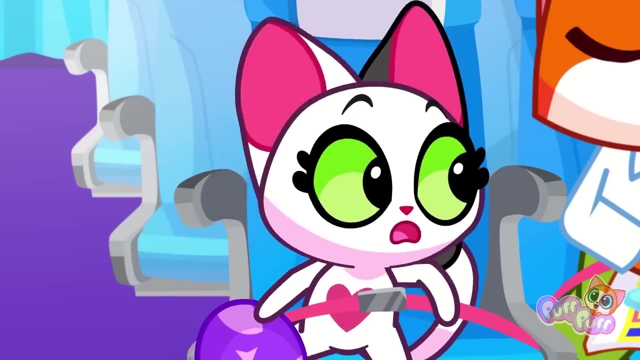 Don't break the line. It's important to keep the line. Baby don't be afraid, Don't be afraid, Baby don't be afraid, Baby don't be afraid, Don't be afraid. It's dangerous. How do I do this? It's dangerous. It's dangerous.